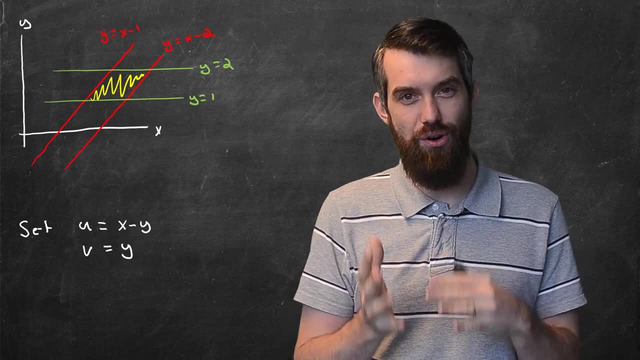 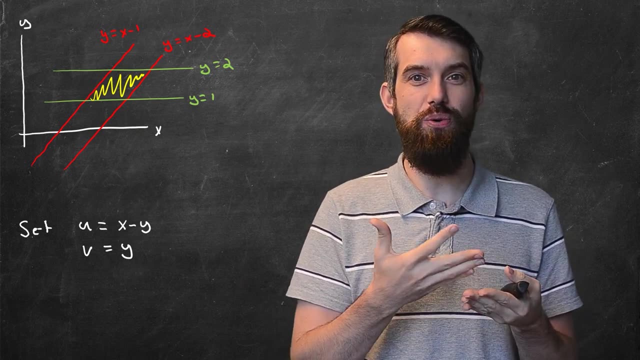 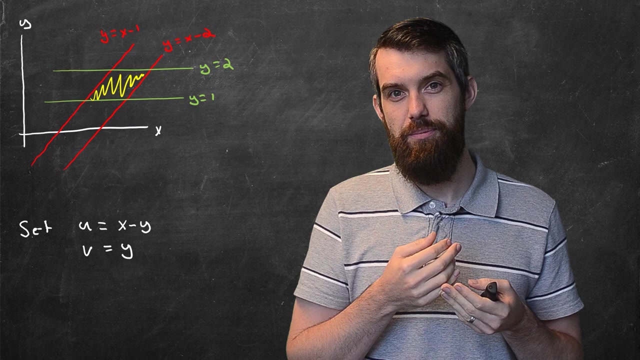 lines, those are perfectly fine, But for the two diagonal lines that are not easily expressed by x equal to a fixed value, if I set u equal to x minus y, then the one line is just, you know, u equal to 1 and the other line is u equal to 2.. These are just constants, Indeed. 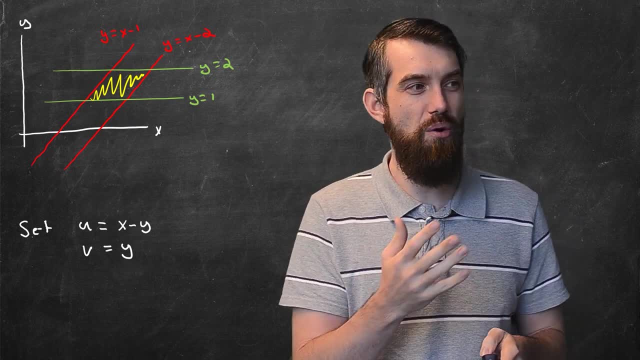 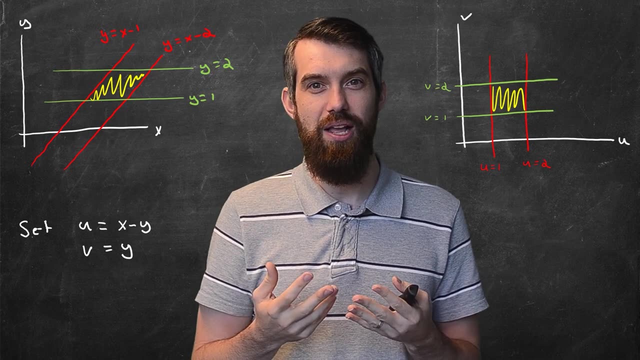 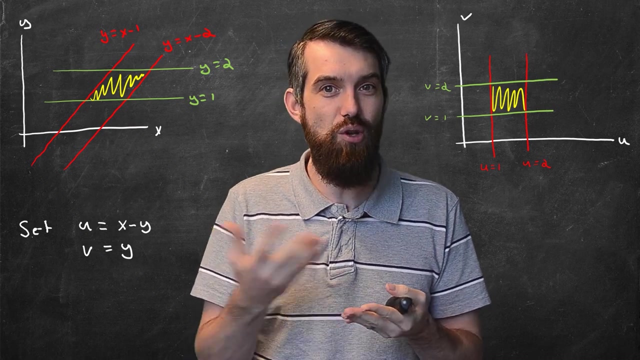 if I tried to draw the exact same region, but now in the uv plane, that is, expressing it in terms of u and v, opposed to x and y, then what I get is just a rectangle. It's just the rectangle where the v values are between 1 and 2 and the u values are between 1 and. 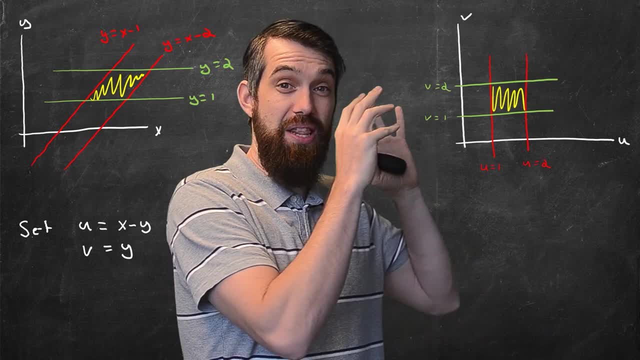 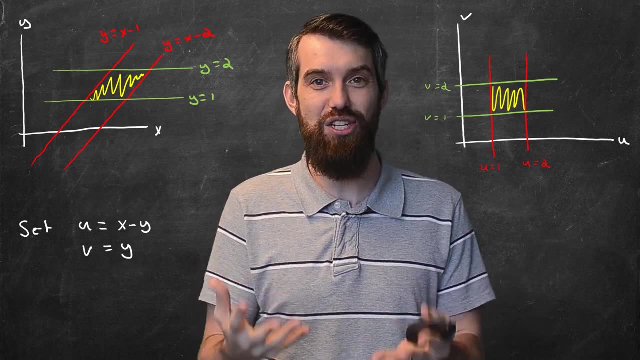 2.. So my plan is that this is going to be way easier to integrate. in this coordinate system, The limits of integration are just going to be 1 and 2 for u and 1 and 2 for v. So how do I actually integrate in some new generic coordinate system? 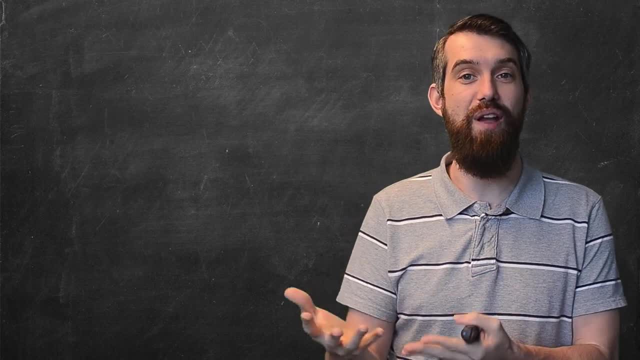 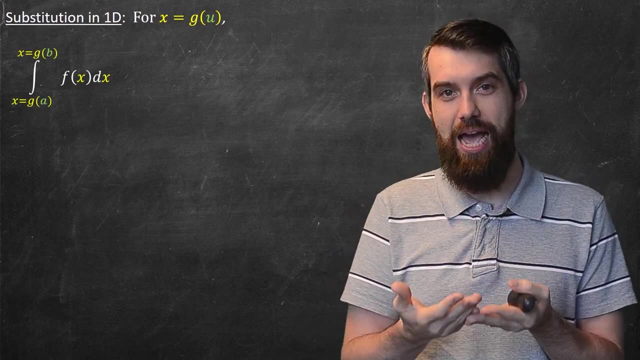 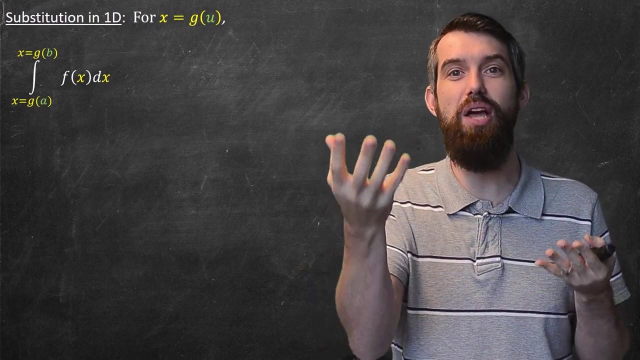 Let's think back to what we used to do for single variable u-substitution. The idea was the following: Suppose I have an integral of some function of x- dx, Then what I can do is take x and write it as some function of a new variable, a new variable u, And then 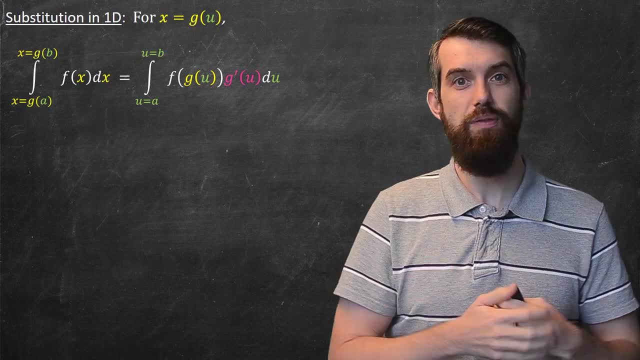 what the u-substitution is going to do is take x and write it as some function of a new variable, a new variable, u, And then what the u-substitution did was: it allows us to rewrite this. This new integral is an integral in terms of u. 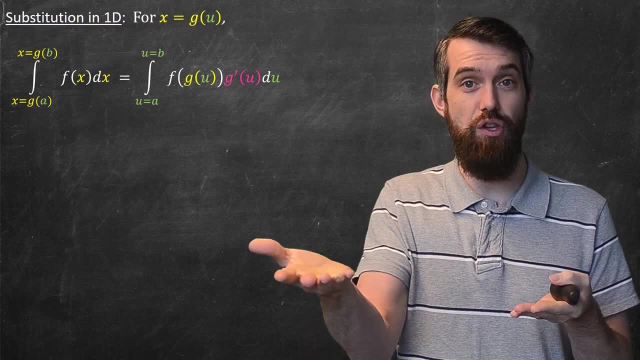 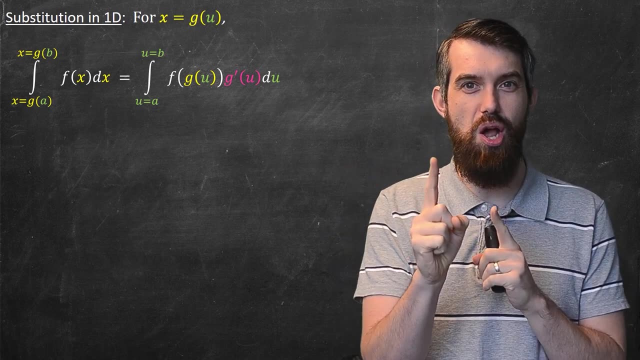 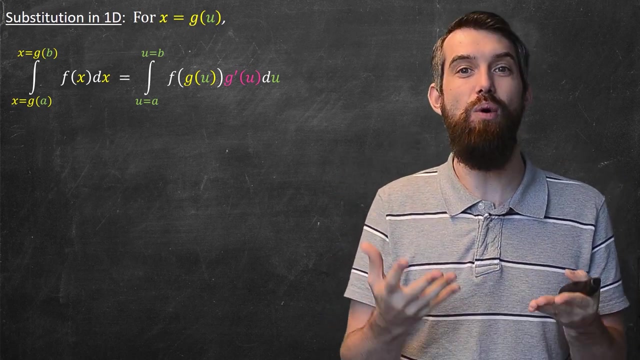 The function of x is now turned into f of g of u, because x is defined to be g of u And the dx transforms into a du. but there's an important point to note: There is also this new factor, this scaling factor, this g prime of u, And that was u-substitution. 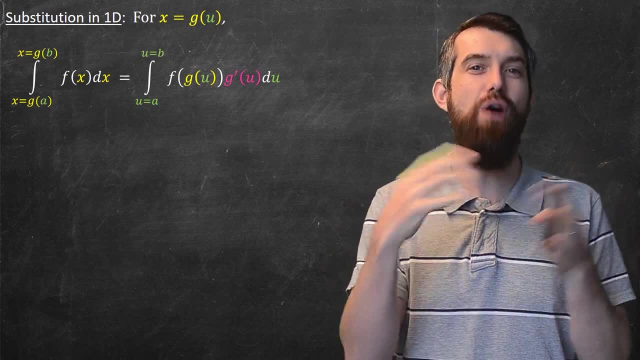 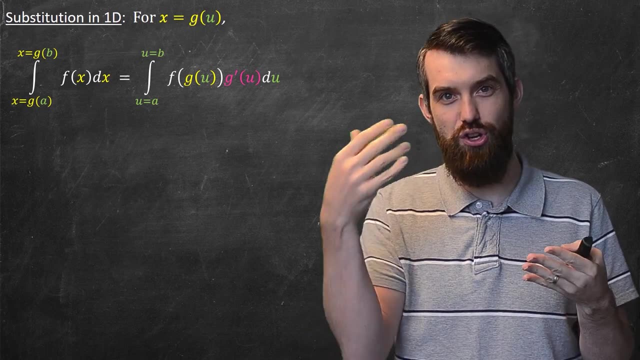 I'll note that this formula may seem exactly backwards to how you would recall it in a single variable calculus. Typically, in single variable calculus you would actually set u to be a function of x, opposed to x being a function of u. It doesn't matter which way. 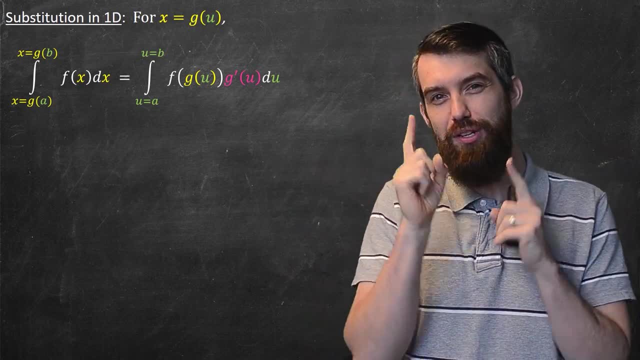 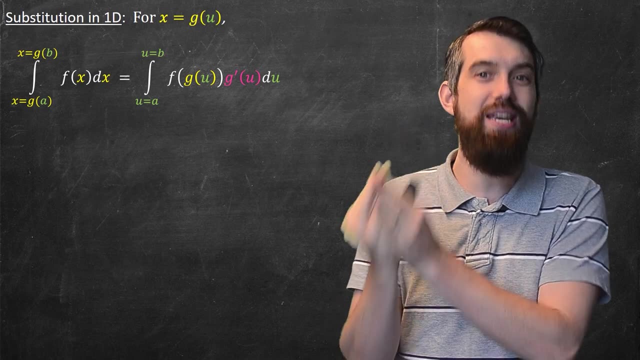 you write it, which you think of as sort of the new variable and the old variable. But I'm going to do it this way because I'm about to have a u and a v And I want to think of the new v as converting the messy xy into a nice u and v-coordinate. So I like this. 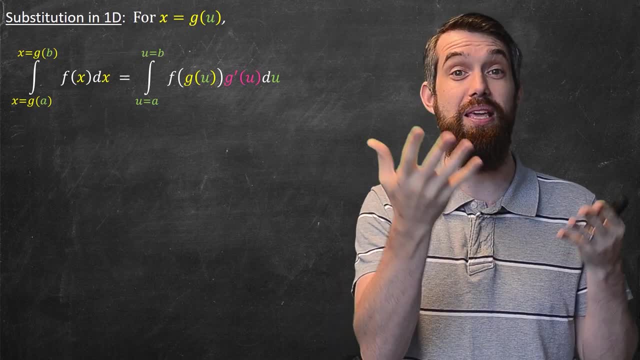 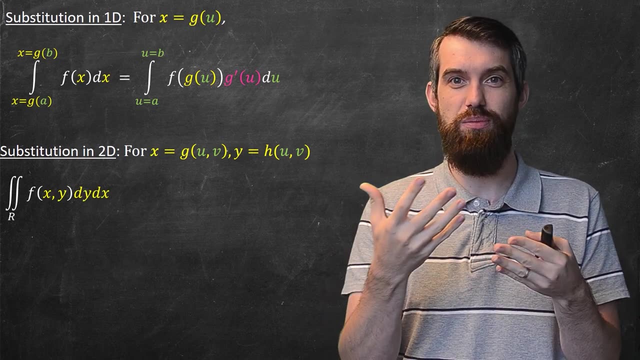 order of presenting it. Nevertheless, let's go and look at what it's going to be in multivariable calculus. Well, you begin sort of much the same way. You have an integral in terms of x and y, and it's integrated over some particular region, And then you say: I'm going to take 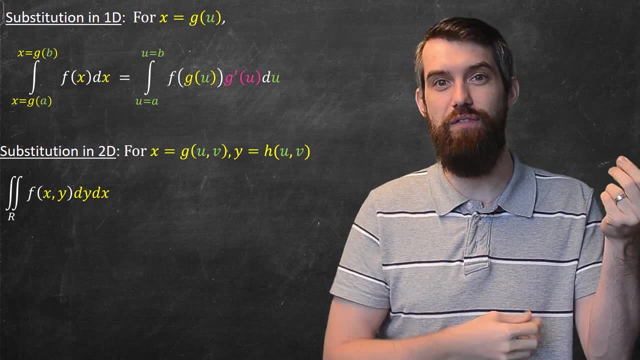 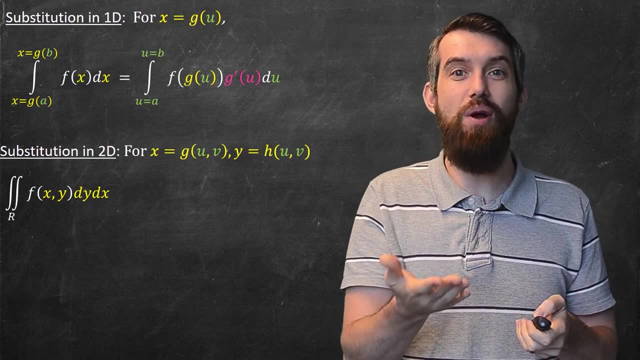 the x and write that in terms of u and v, some function g of u and v. And I'm going to take the y and write that in terms of u and v, some function h of u and v. Then, if I plug this all in, I want to get an integral with respect to u and v. Well, the function. 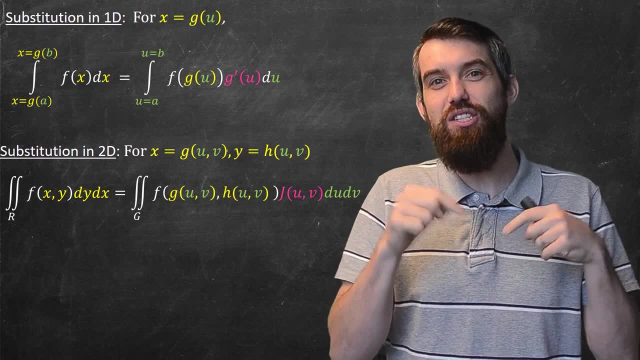 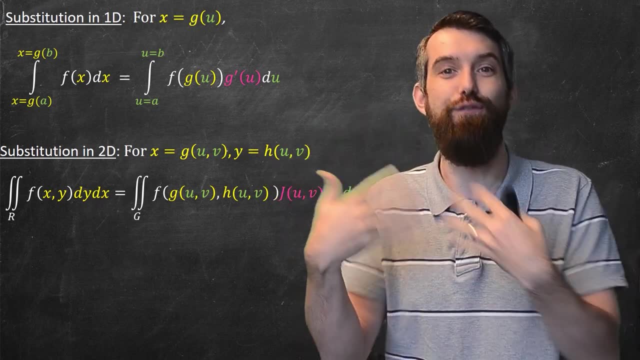 evaluates now in terms of u and v. The limits of integration are no longer the same. They are no longer the region r, Now we call it the region g. It's what happens when you transform under these equations And then the dx, dy transforms into a, du, dv, But just. 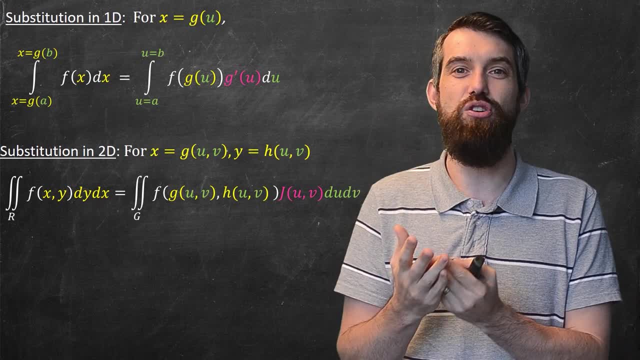 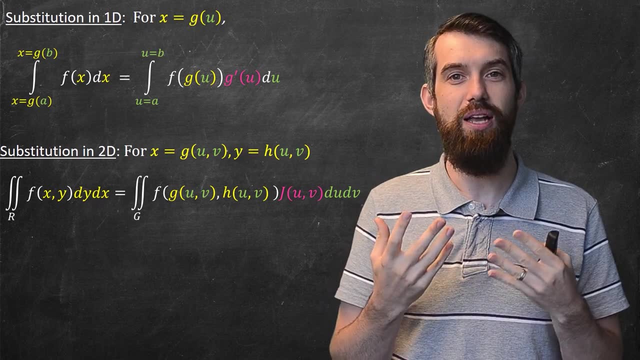 like in the single variable case, you have to have a multiplicative factor. We're going to call this multiplicative factor no longer g prime, We call it j of u and v. Here j is called j for the Jacobian. At the end of the video I'm going to talk about the intuition. 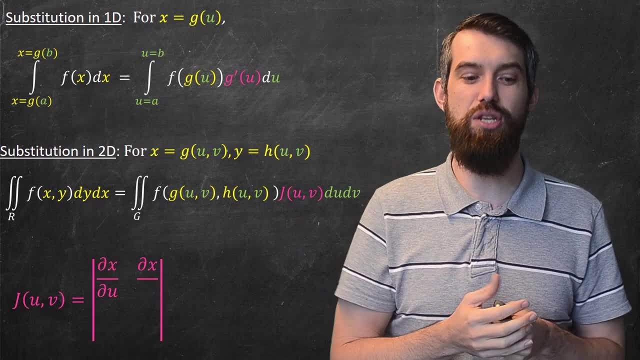 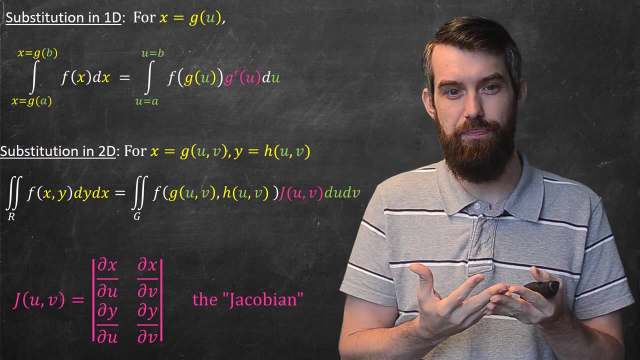 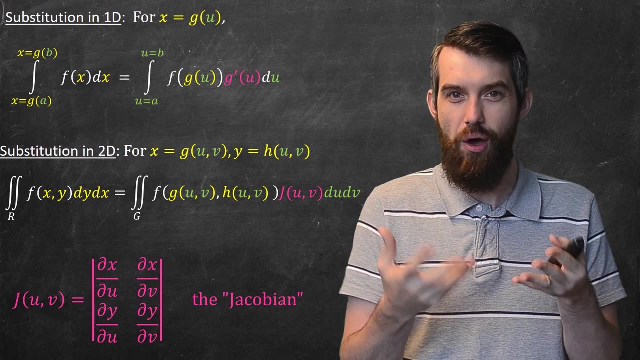 of how to come up, But for now I'm just going to state it. j of u and v, the Jacobian is just the determinant of a particular matrix, a matrix of partial derivatives, And the idea here is that this represents the scaling factor from when you shift your areas. thought of in terms of the 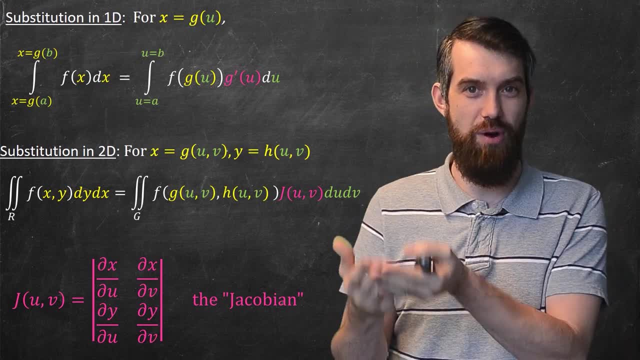 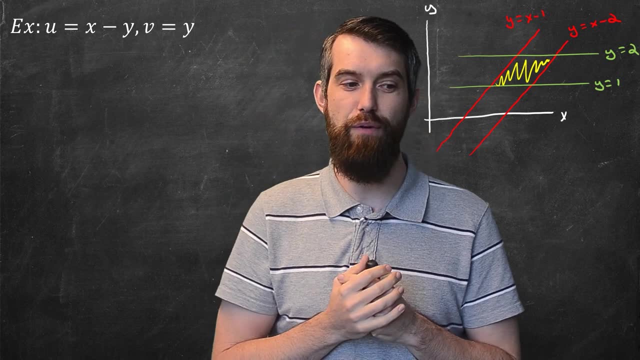 xy coordinate system to being areas in the uv coordinate system. You need to get a scaling factor, and this j gives you that scaling factor. All right, so let's look at the example that we had before, where our u was equal to the. 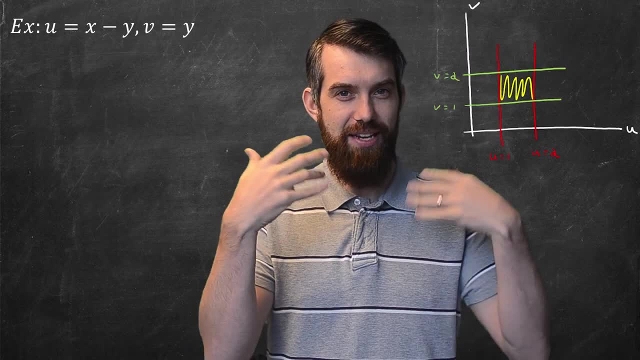 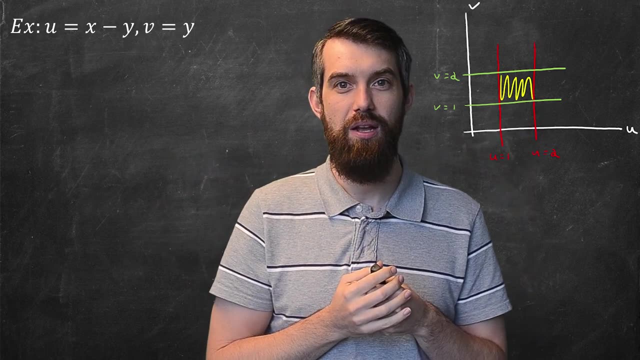 x minus y and our v was just equal to y. And then, if I take that exact same region, I now represent it in the uv coordinate system and it looks a lot nicer. First thing I want to do is try to write it in the way that's compatible with my formulas, where I had x. 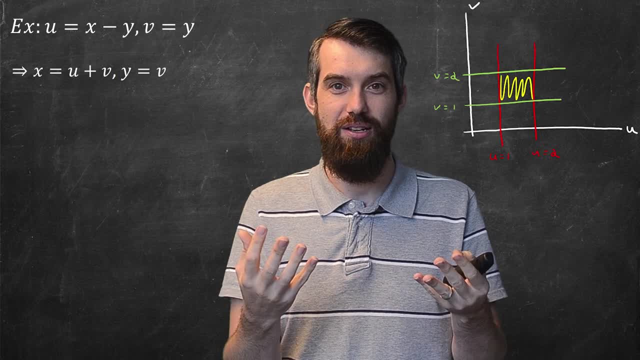 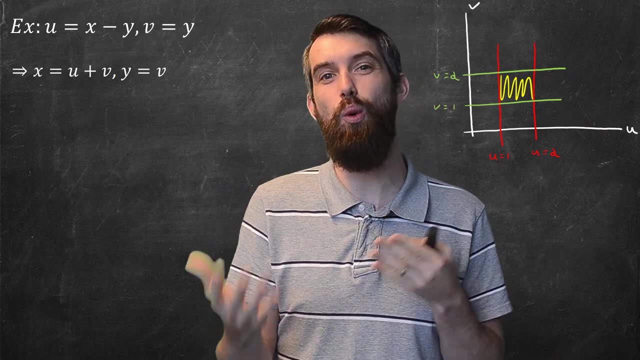 as a function of u and v and y as a function of u and v. So I'm just going to take these formulas, I'm just going to rewrite them in that way And if I do that, of course y is equal to v is the same thing as v equal to y. I plug that in and I get x is equal to. 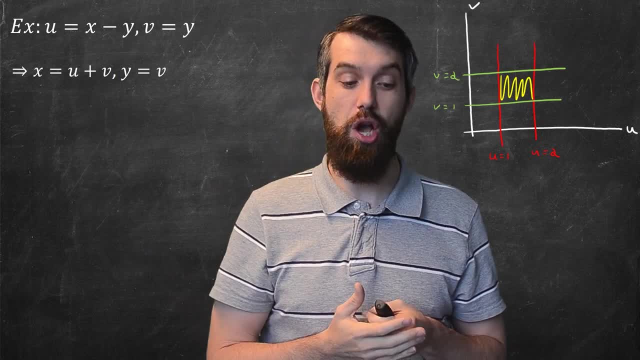 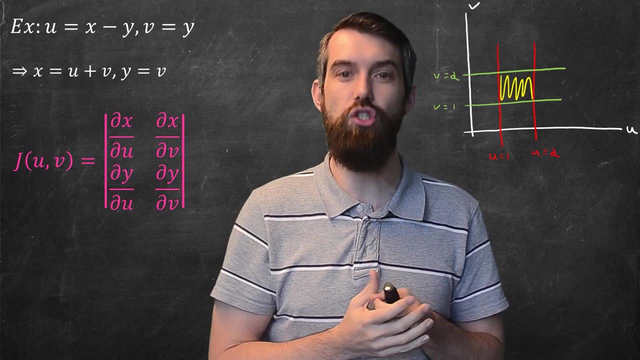 u plus v. All right, so let's compute out that Jacobian, this determinant. Well, most of these partials are straightforward, which the partial of x with respect to u, well, is just 1, and so on. So I can compute what these are going to be. It's just the determinant. 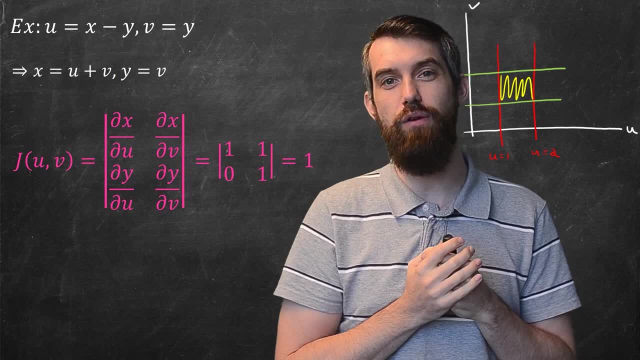 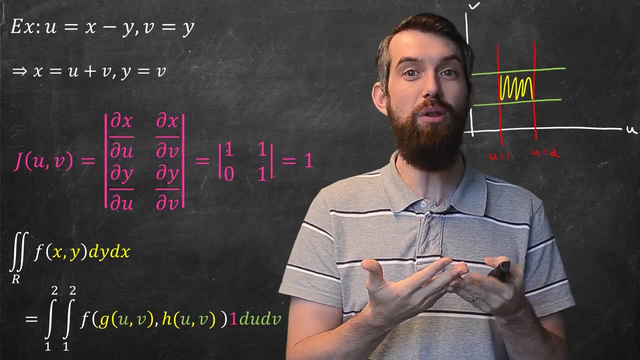 of the matrix 1,, 1,, 0,, 1,, and that's just equal to the value of 1.. So, in this case, the Jacobian is just multiplied by 1.. So here then is my final formula: The double. 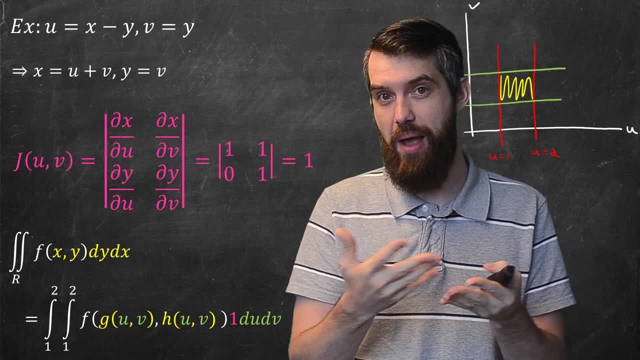 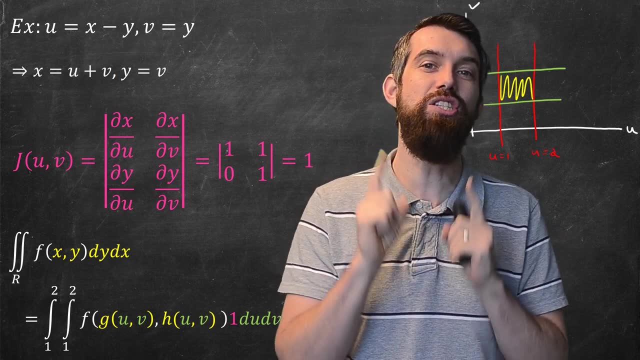 interval over the original region, the sort of parallelogram one. if I take that region and integrate some function of x and y over it, it's the same thing as the much simpler region, the region in the uv coordinate system, where the u integral just goes between: 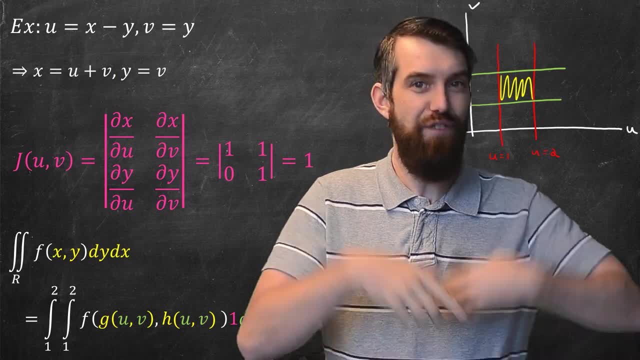 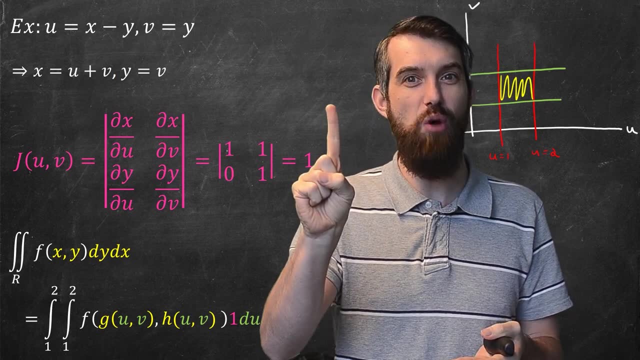 1 and 2, and the v integral just goes between 1 and 2.. The function, whatever it is, I haven't told you would be represented now in terms of u and v. You multiply by that 1 for the Jacobian and then you get your result. after you integrate with respect to u and v, You 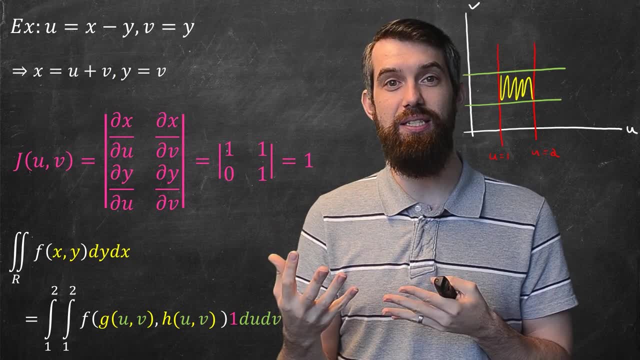 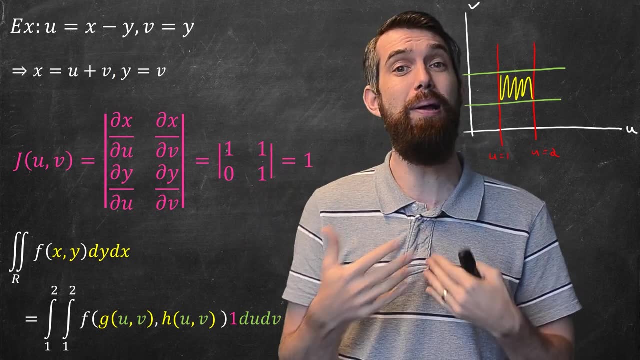 might want to do this transformation of variables for multiple reasons. It might be that your region is really messy and you can transform it into a much nicer region with the substitution. or it might be that your integrand is really messy and you don't. 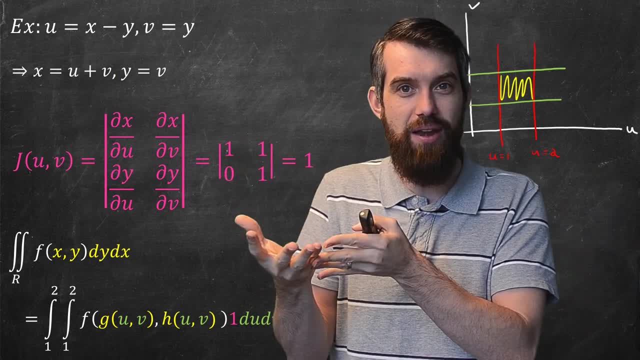 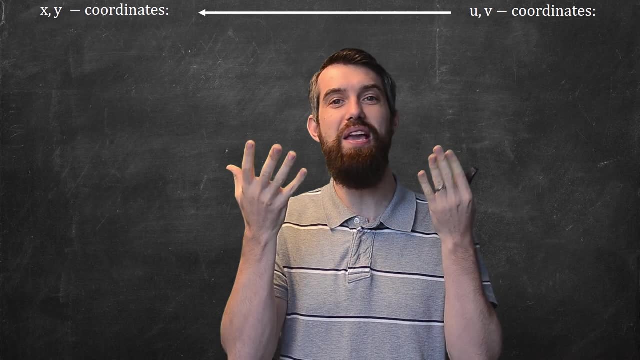 know how to integrate that and then with the substitution, you can now integrate the integrand There's multiple reasons why you might wish to do a change of variables. Final thing I want to talk about in this video is motivate the j of u and v, the Jacobian. 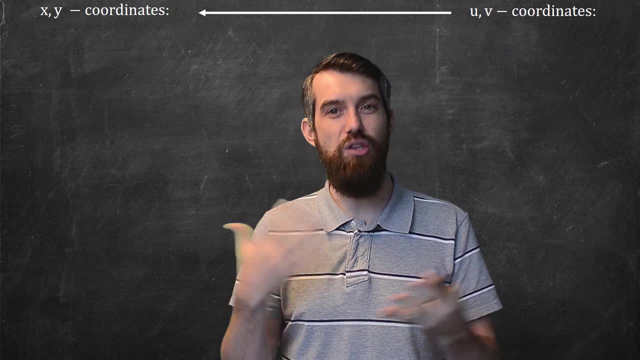 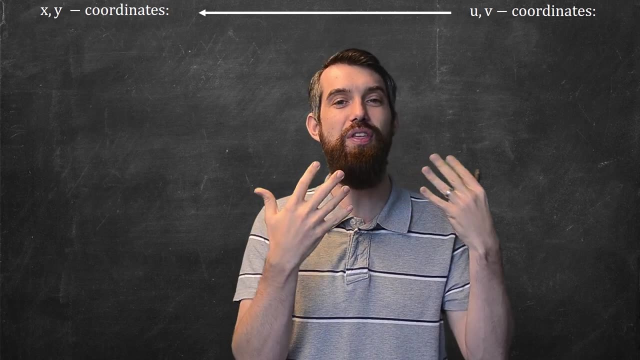 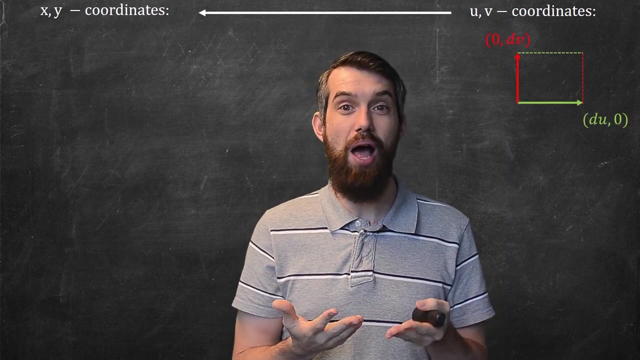 Why was that the case? So I want to imagine that I'm in the uv coordinate system and I'm going to transform a little region, A little area in the uv coordinate system into the xy coordinate system. That is, imagine I just have a little rectangle. This is a rectangle and it can be described by having 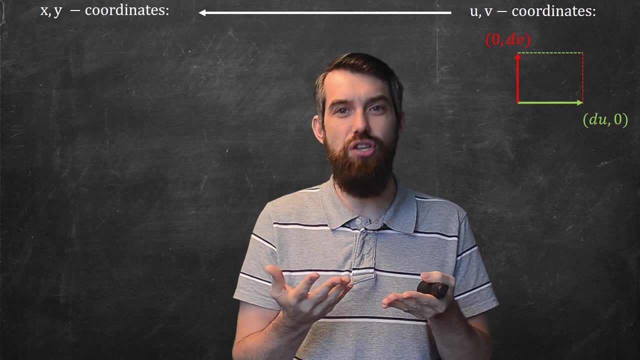 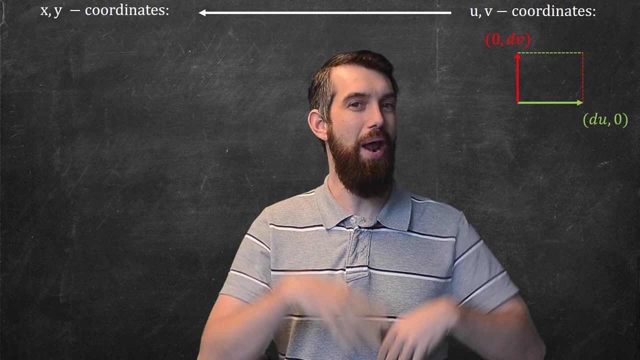 two different vectors. One vector is a little change in u and no change in v, and the other one consists of no change in u and a little change in v. When I integrate, of course, I take a region- I think of breaking it up into a bunch of little regions. So in the 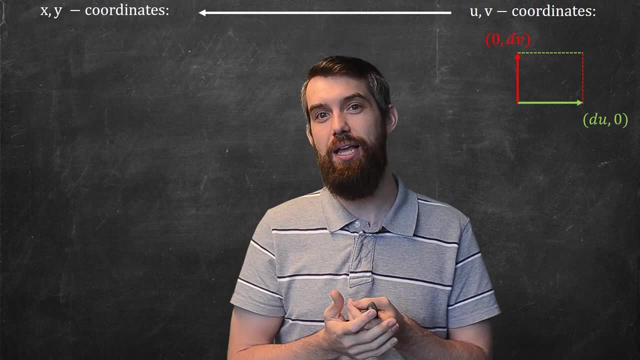 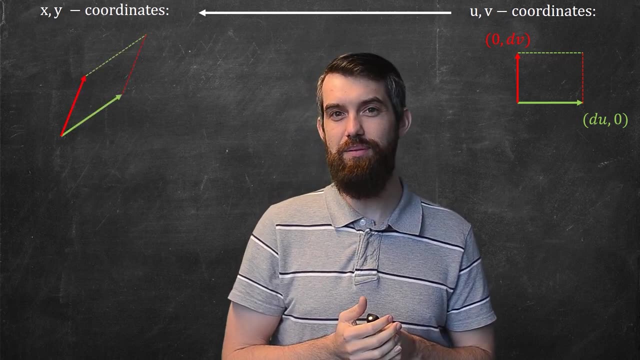 uv coordinate system. these little regions are simple, They're just little rectangles. But let's see what this little region looks like all the way back in the xy coordinate system. Indeed, this green arrow goes somewhere, the red arrow goes somewhere, and whatever. 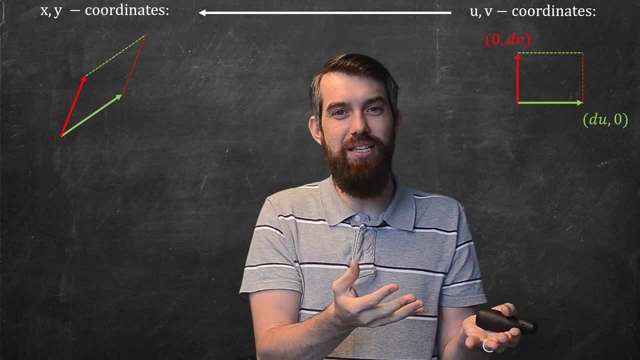 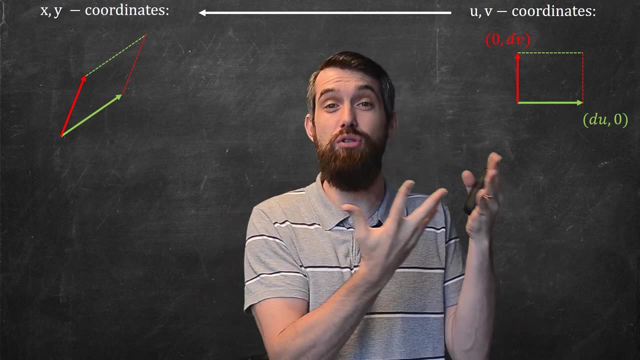 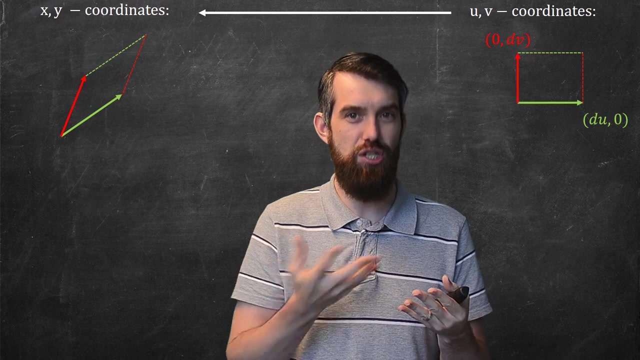 you get, defines a parallelogram As in the original square defined by these two vectors, transforms into a parallelogram defined by wherever those two vectors end up. But where do they end up? Well, if you think of the green vector, as the result of just first, a 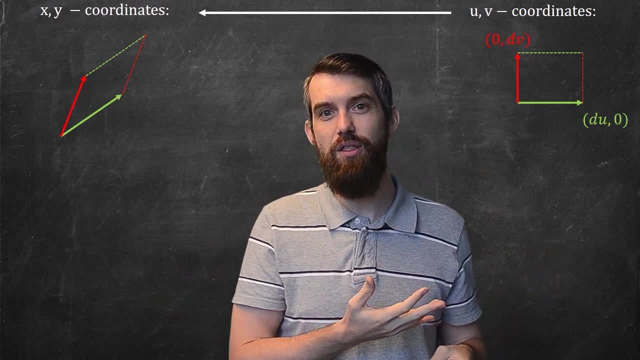 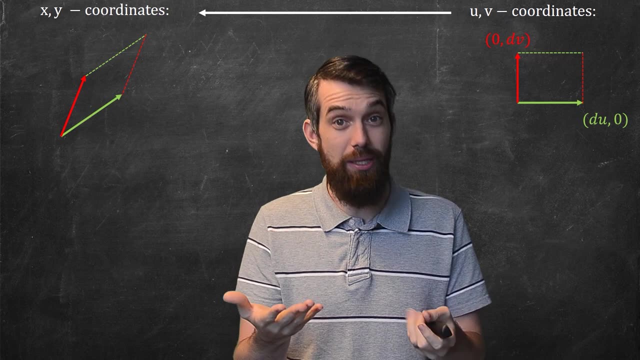 small nudge in u and then you transform it into x and y. then the result you get: Well, what change in x do you get? It's the resulting change from nudging the u a little bit, and in other words, what you get is a change in x with respect to u, x And likewise. 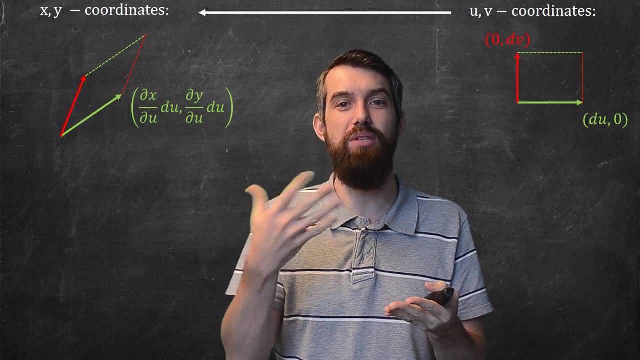 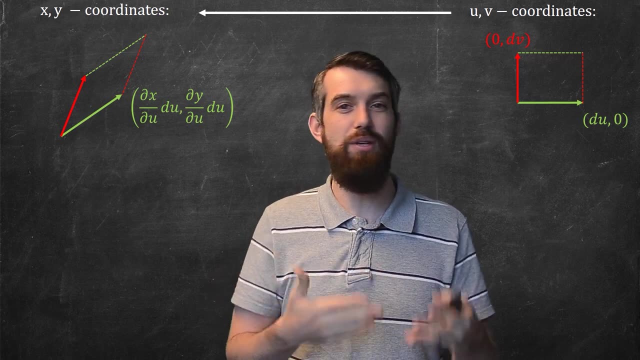 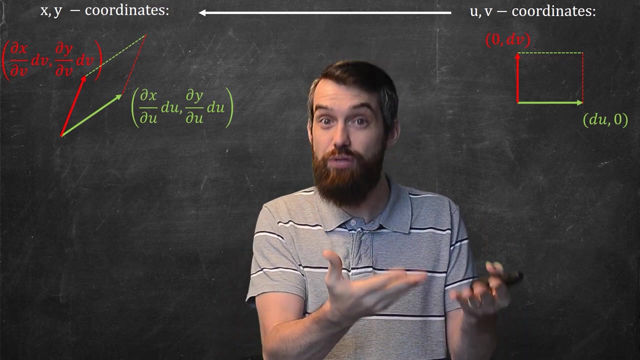 for y. It's the partial of y with respect to u, x, entren. These are the little nudges in the x and y direction that result from nudging u a little bit. similar kind of construct. The nudge in the x direction is just the change in x. 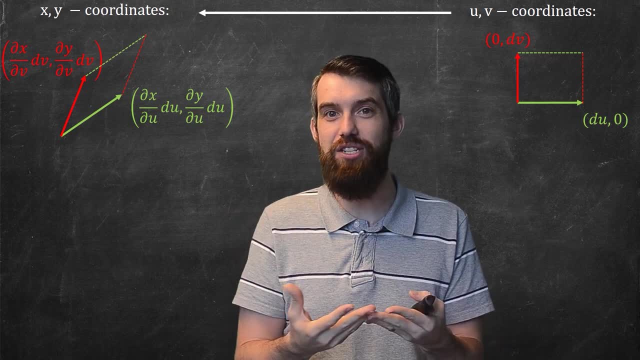 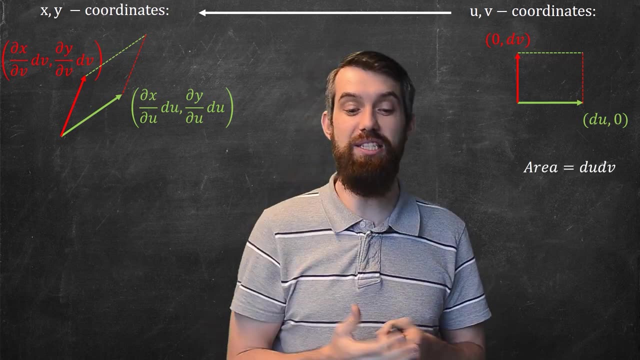 with respect to v times, this dv and the change in the y direction is the change in y with respect to this v dv. Now back in the original UV coordinate system, the area was easy to express: It was just du times dv. So if you're a big region, you 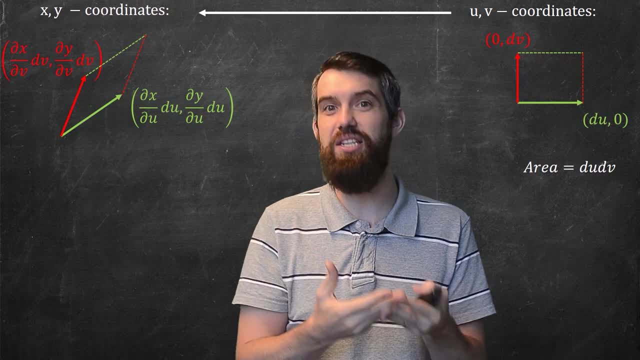 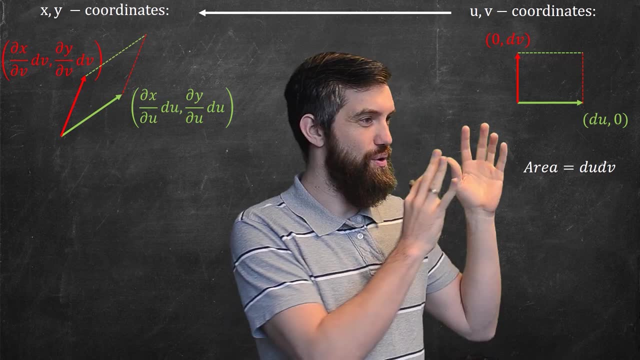 make it a bunch of little rectangles. These little rectangles have areas du, dv, Exactly what we've seen when we defined double integration. But now, if I ask the area for this same region but then map back into the x-y coordinate system, well, 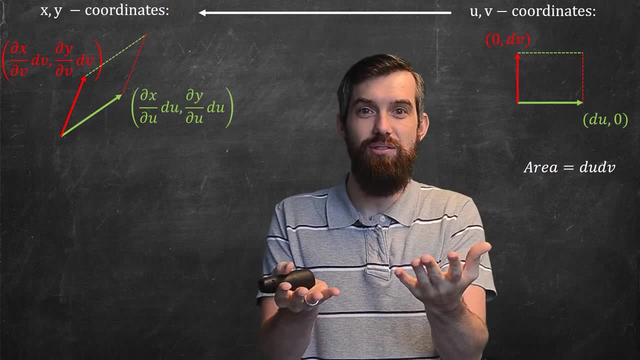 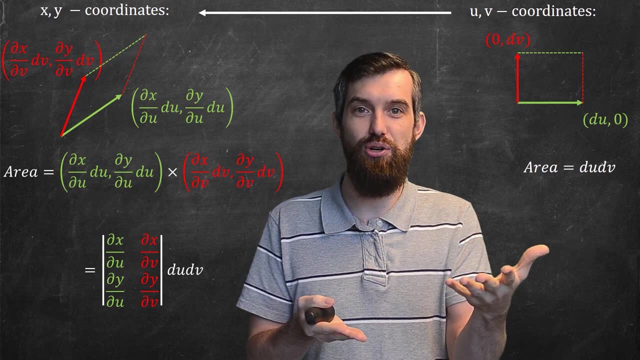 area of the parallelogram is a cross product. So what is the area of this new parallelogram? Well, it's just going to be the cross product of these two little vectors, and the cross product of those two different vectors is the determinant. 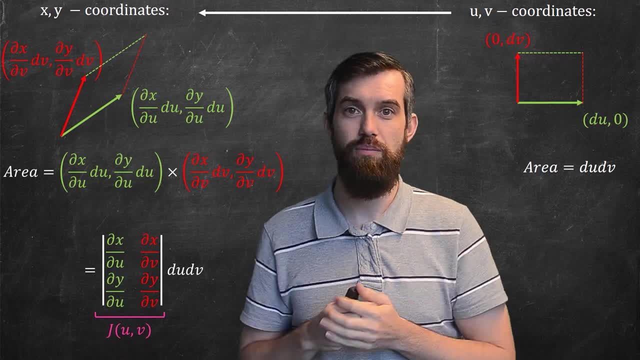 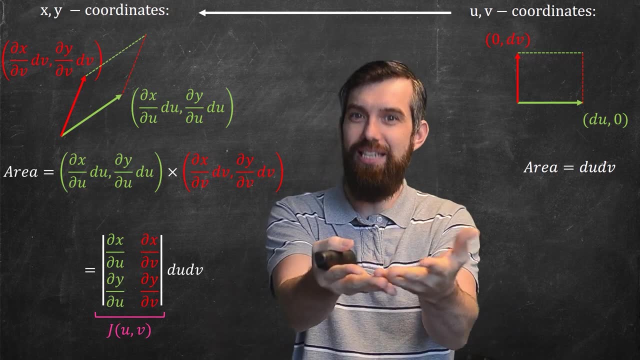 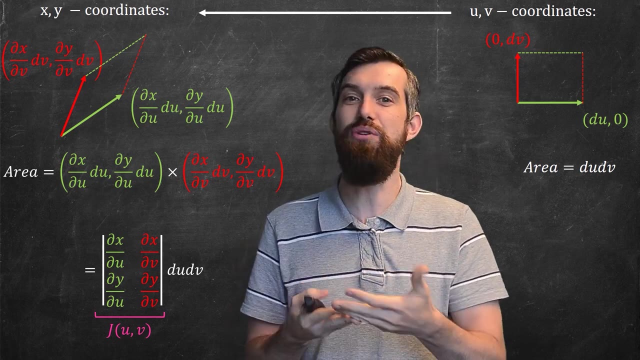 that we've seen before. Indeed, this is nothing but the Jacobian. So what does the Jacobian represent? It says, if you take a region in UV, a little area in UV, you transform it into the x-y coordinate system system. well, you get a multiplicative factor on their areas. The du dv transforms to this matrix. 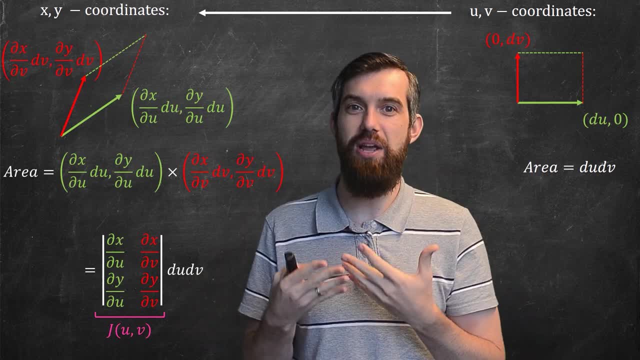 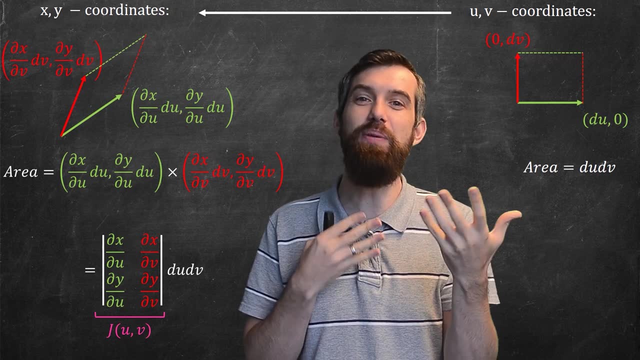 times a, du, dv. So if you're going to integrate with respect to these new coordinate systems, that's fine, that's great, it's easy, but you have to bring along this multiplicative factor, this j of u and v. If you have a question about this video, leave it down in the comments below.